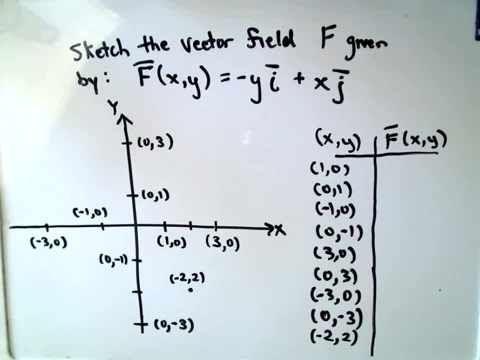 Okay, so kind of a basic example here, nothing too complicated, Kind of a typical type of problem that you'll see. So I'm going to sketch the vector field F given by. I should put a little bar over my F here too to emphasize it's a vector function. 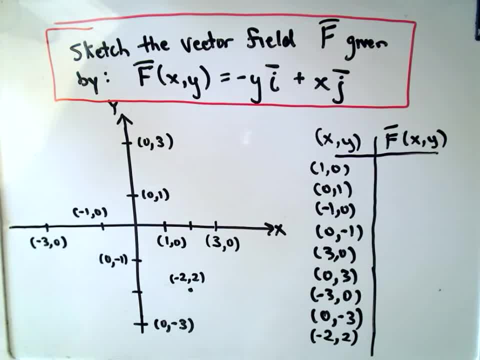 Given by negative YI plus XJ will be the formula. So I've got my little X and Y axis. I've plotted a bunch of points- you know kind of arbitrary points- And I've made a little list of all the points. 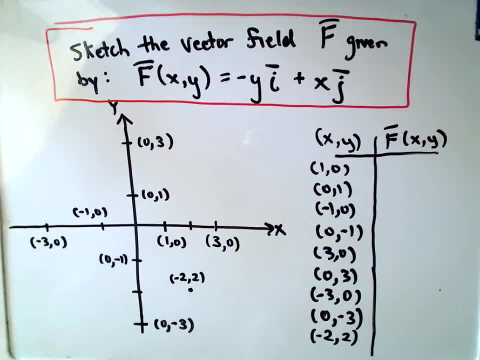 So I'm just plotting points at random just to help me get an idea about what this vector field will look like. So quite a few here. I'll do the first couple pretty slowly and then a little faster Again. this is something you wouldn't do by hand, much for sure. now. 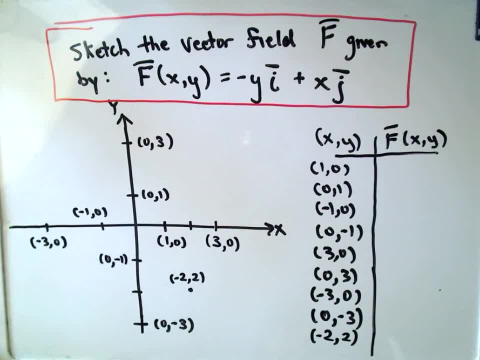 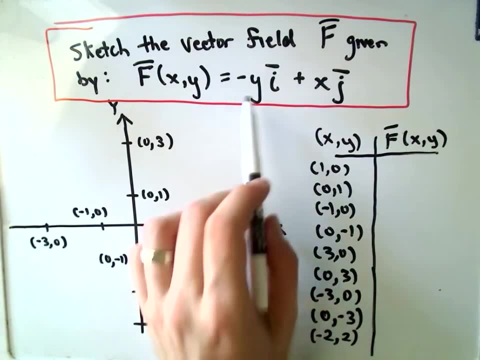 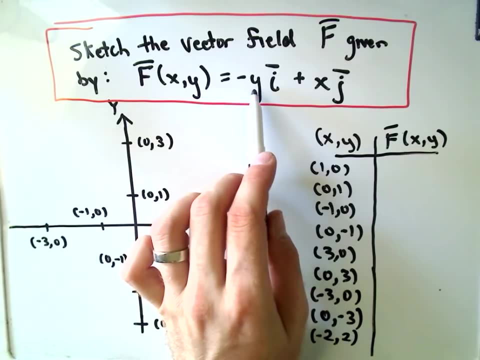 You would have a computer, you know, sketch a bunch of these. But just to give you the basic idea, Suppose we want to sketch the vector that's associated with the point. Well, if we plug into our formula, notice that the X value goes with the J component and the Y value goes with the I component. 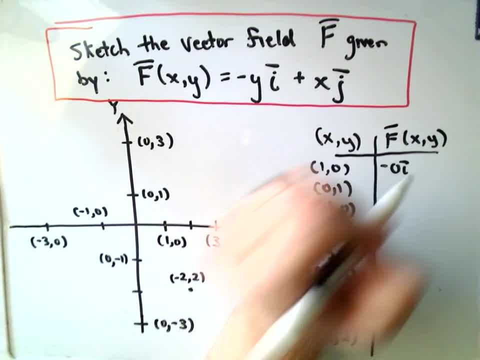 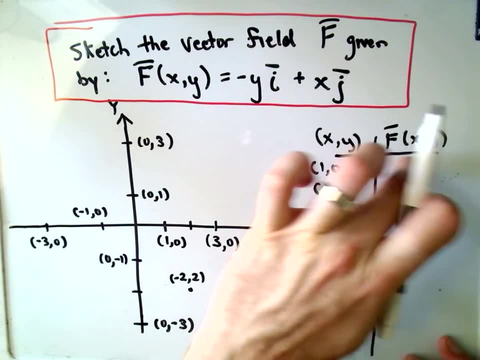 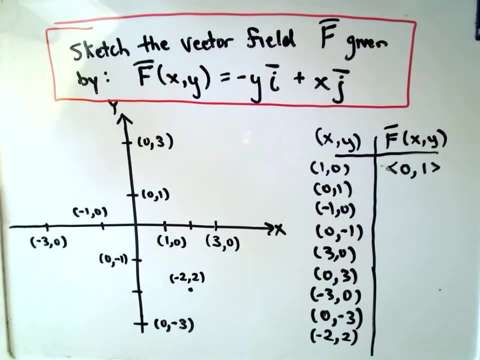 So we would get- It looks like to me- plus 1J, And we can simply rewrite that as 0, 1 using our little brackets, our vector notation. Likewise, I'm going to do maybe the first four real quick. 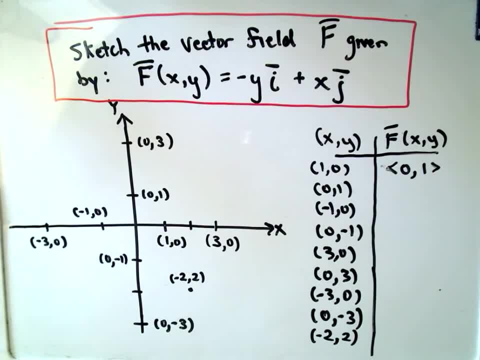 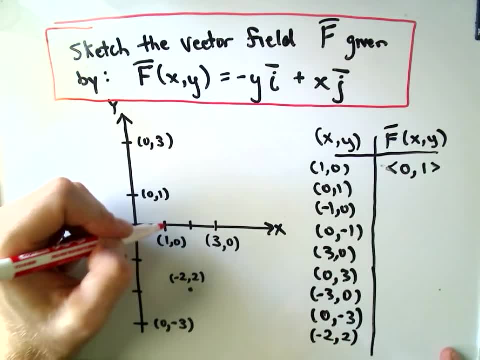 Notice if we plug. Well, let's go ahead and do this one real quick. So it says at. it says the vector associated with the point is going to be the vector. And remember that means it's just a vector that doesn't move left or right but just goes up. 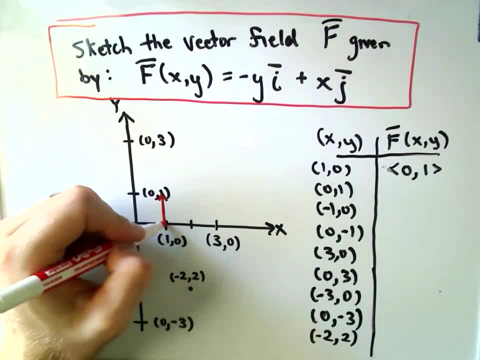 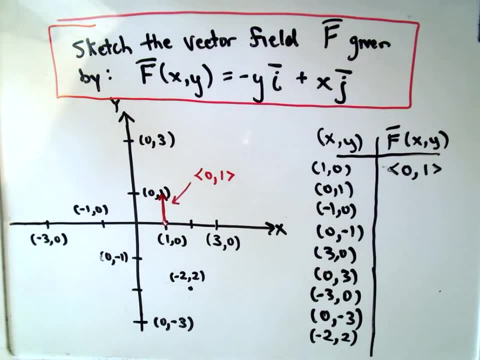 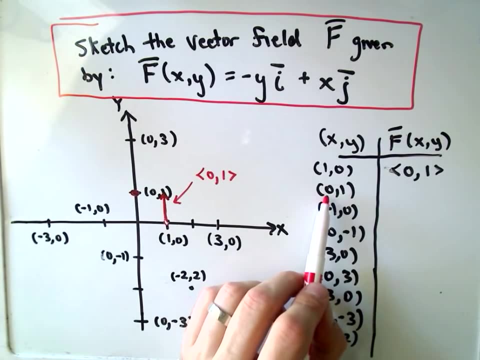 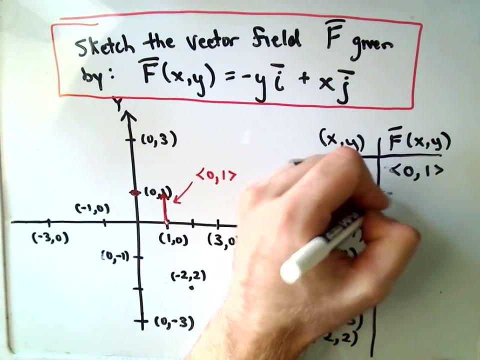 It points Directly upwards and it goes out one unit. So that would be the vector. Likewise, if we find the vector associated with the point, Well, again, if we plug 0 in for X and 1 in for Y, we would get. 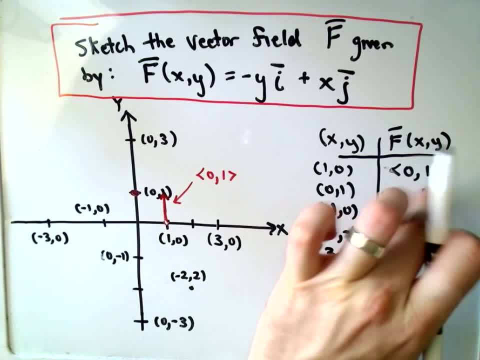 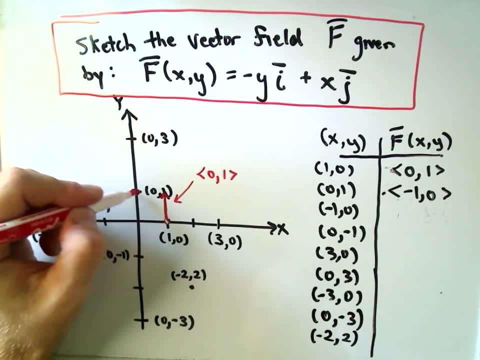 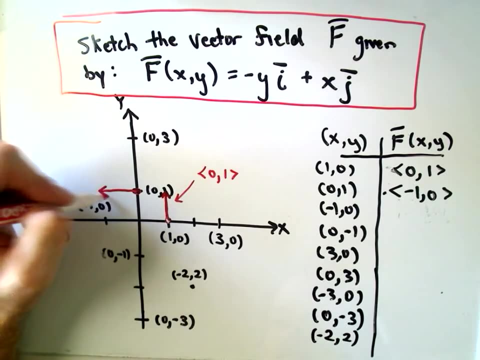 And if we simplify that again, I like to use the little bracket notation We would get. So it says at the point. it says your vector is pointing one unit to the left but it doesn't go at all up or down. So my vector at the point would look like this vector: 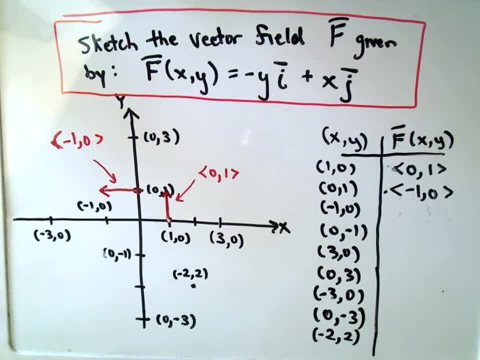 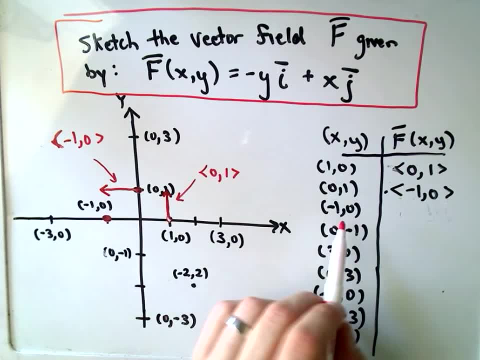 So it would be the vector, And really this is all you're doing. You're just plotting a whole lot of points. At notice, if you plug that in, So if we plug for the X coordinate. So I'm just going to start using my bracket notation. 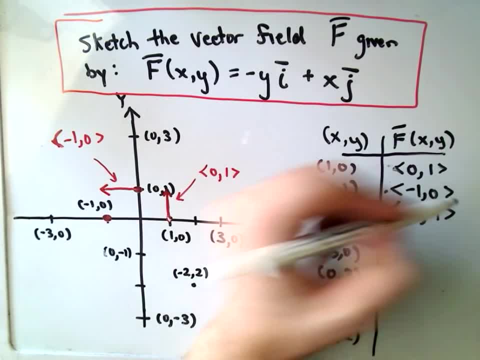 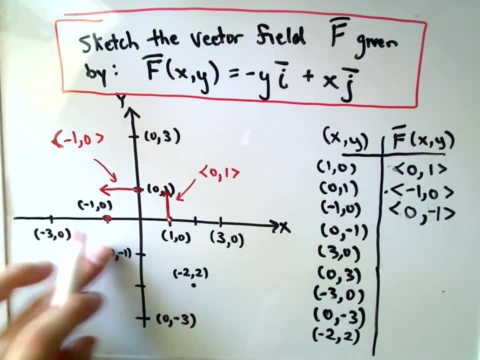 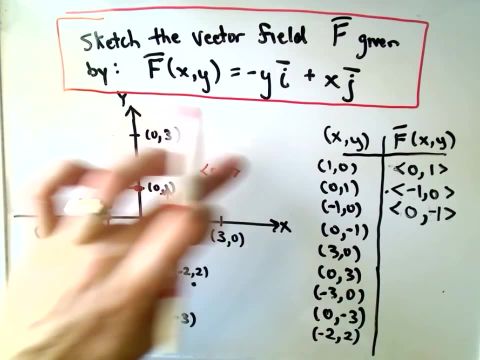 So if we plug for the X coordinate, we'll get. If we plug for the Y coordinate, we'll get, And notice this is just going to be a vector pointing one unit down. So let me try not to clutter up my picture here too much. 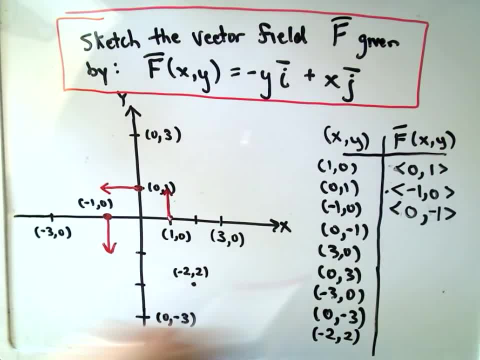 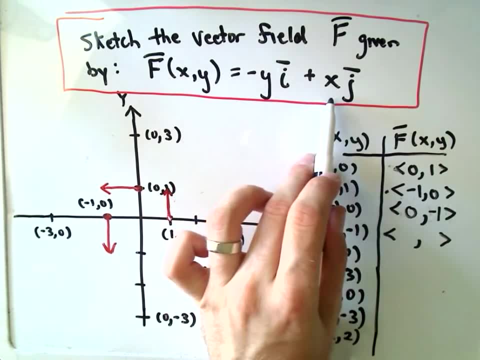 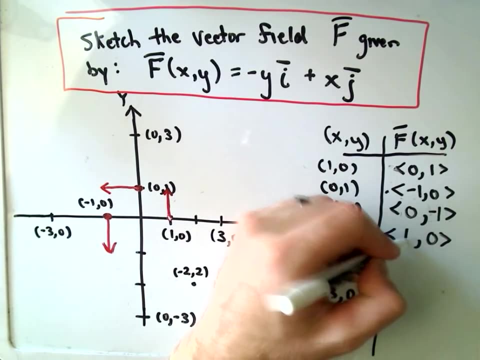 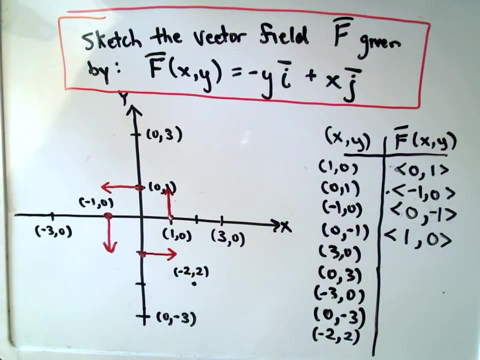 And likewise we could plug in. So If I plug 0 in for X into my formula, I'll get 0 out for the J component. If I plug in for the Y component, I'll get- And that's going to be a vector just pointing one unit to the right. 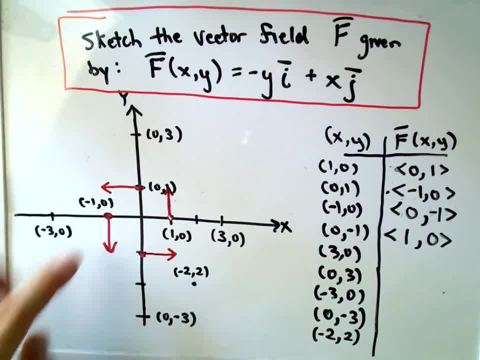 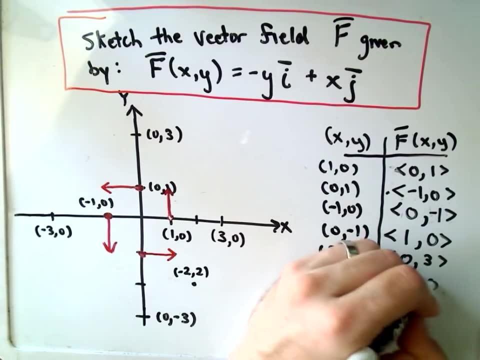 So there's a few points associated with So a few vectors associated with four different points. I think you can kind of go back and check: If you plug in, we're going to get, If we plug in, we're going to get. 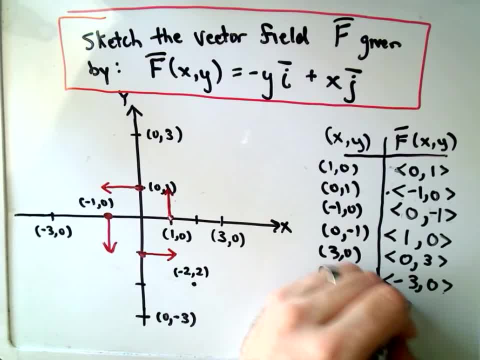 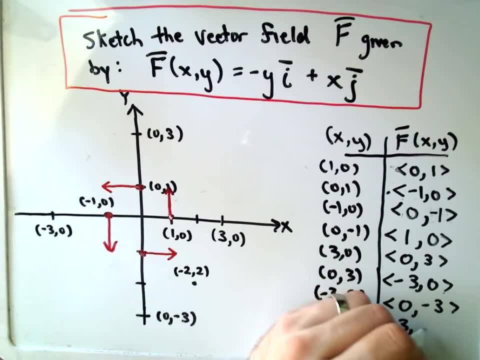 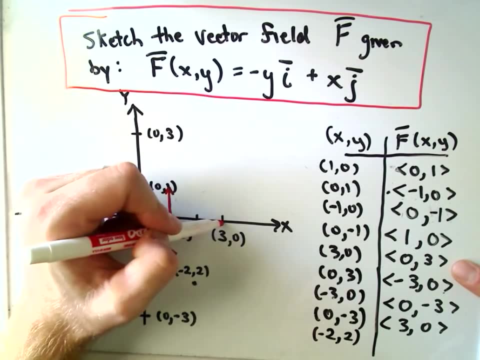 If we plug in we're going to get, And if we plug in we're going to get as our vectors. So it says at. It says you're going to get a vector that's pointing three units upwards. So that's supposed to be. 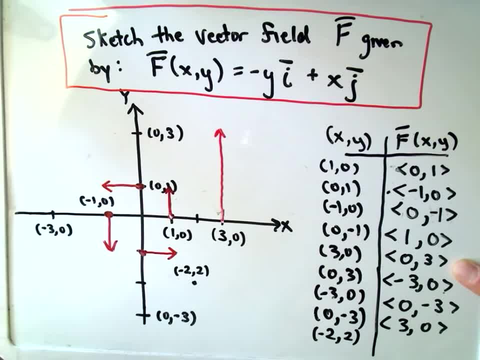 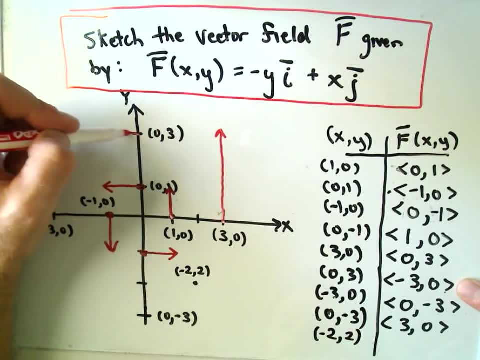 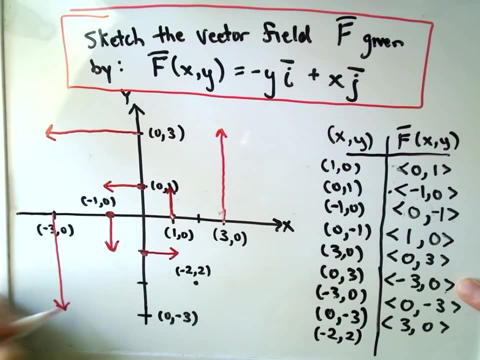 It's terrible. It's supposed to be going straight up. three units At the. It says it's pointing three units to the left and no units. It doesn't move at all up or down. Likewise, at will be down here. It'll be pointing down. 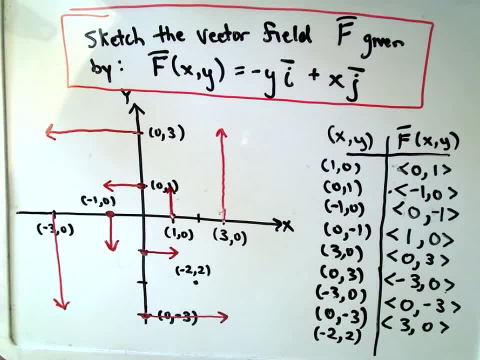 And at It'll be pointing to the right three units. I've got one more little point in there. I plugged in just to give me one other point. Last but not least, So again this is very tedious stuff. If you plug in for we'll get. 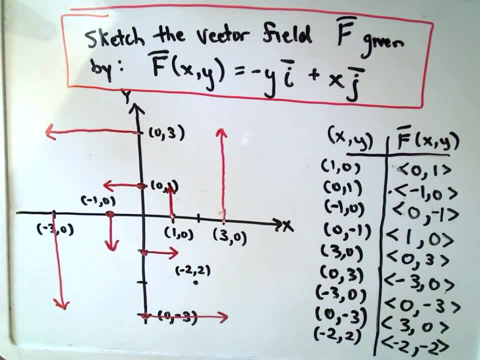 If we plug in for we'll also get Whoops. This is totally the wrong point. Terrible Dyslexic here. How about I'm doing the same thing? How about That'll be a little bit better here? 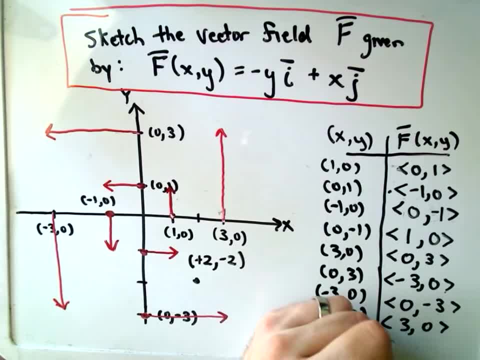 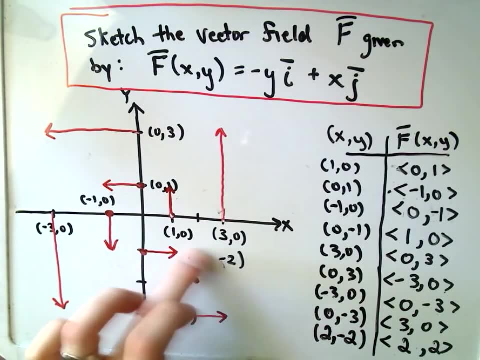 Okay, So if we plug in the point, So if we plug in for the y coordinate, we'll get. If we plug in for the x coordinate, we'll get. And again, that's a vector pointing two units to the right and two units up. 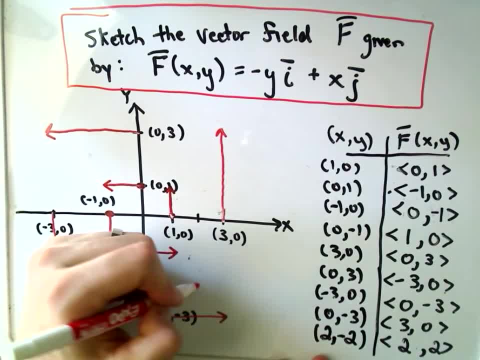 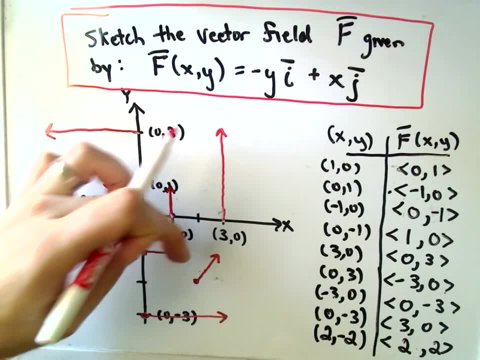 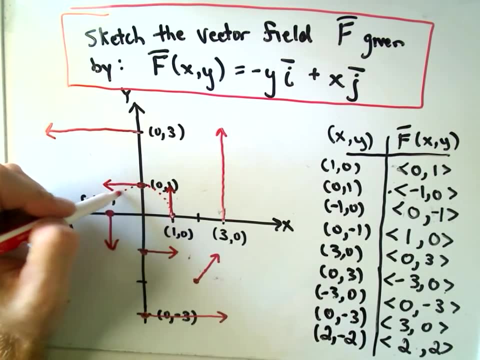 So that vector would look something like that. It should be longer than the first set I did, but not as big as the outside ones. I think to me what's kind of looking like it's going on here. it kind of almost reminds me of maybe like you know, maybe this is. it's almost like a vortex or something like that. 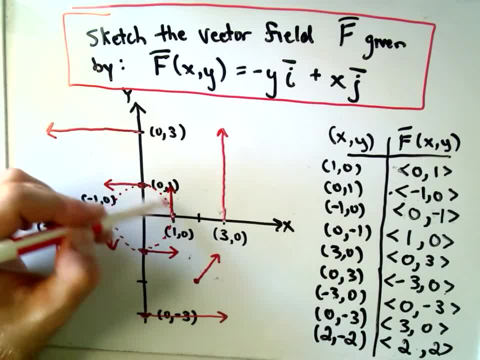 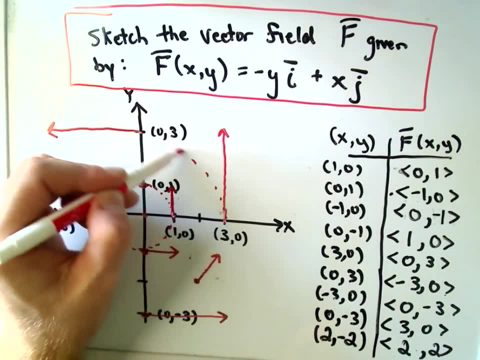 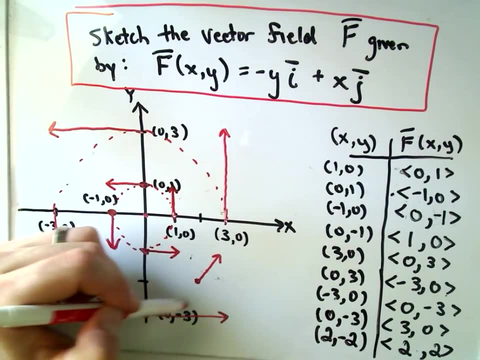 Maybe you're looking from the top. So the stuff on the inside that's maybe spinning around the origin, it doesn't have to travel quite as fast. If there was, you know, imagine, like a solid disk or something of that nature, If the particle is traveling on, you know, further out on the disk, obviously the force on it is going to be much higher as it spins around that center. 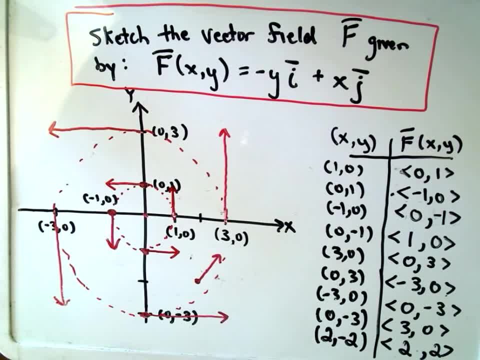 So to me just kind of a little conceptual link between maybe what this vector field could be useful for. But again, generically all a vector field is: take a point, you've got a formula, calculate the corresponding vector, make a pretty picture and hopefully it'll give you some insight into what's going on. 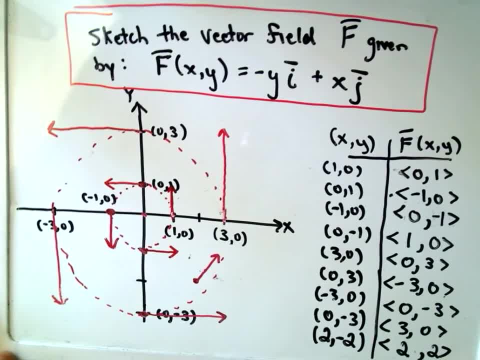 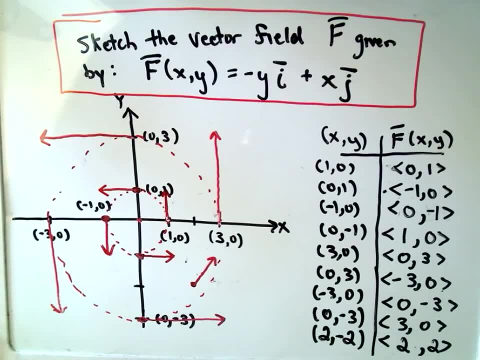 And obviously depends on whatever physical situation you're in. But all right, sorry about my point being thrown off there at the beginning. Silly mistake, but it happens. So if you have any questions or comments, as always, feel free to post them. 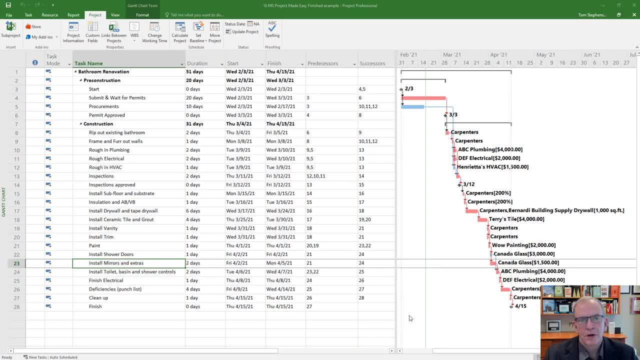 Hi, I'm Tom Stevenson and welcome to MS Project Made Easy. I'm a professor of Construction Management at George Brown College in Toronto and I've been teaching this a long time and I've been doing a lot of things with industry professionals in the construction sector with Microsoft Project. 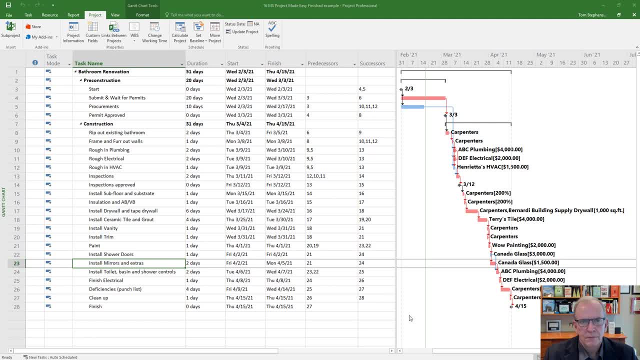 And one of the things I realized is that you can use Microsoft Project for pretty much any kind of project that you may be thinking about. So this is not going to be a series about construction projects necessarily, although I think I'll use a bathroom renovation as an example, But you know. 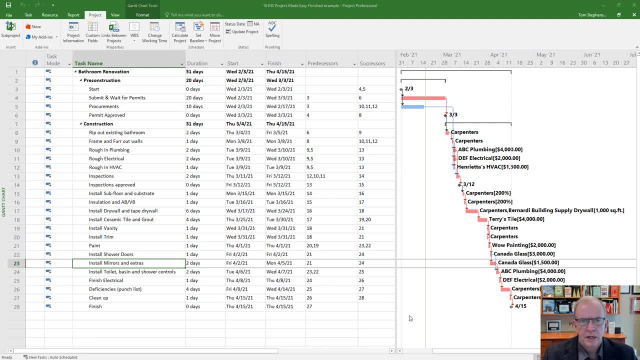 if you want to plan a wedding, if you want to plan some sort of project that maybe even you have at home or at the office. it's a fairly simple tool to use and you can use it to different levels of complexity. That's the other thing. You don't have to go the full nine yards with it, adding resources.